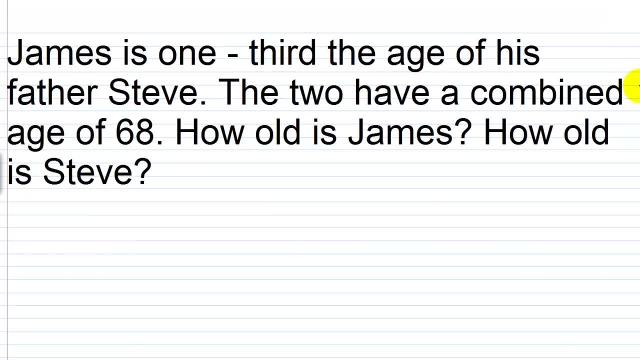 first problem here: It tells us that James is one-third the age of his father, Steve. The two have a combined age of 68 and we want to know how old is James, how old is Steve? So what are we being asked to find? We're being asked to find how old is James and how. 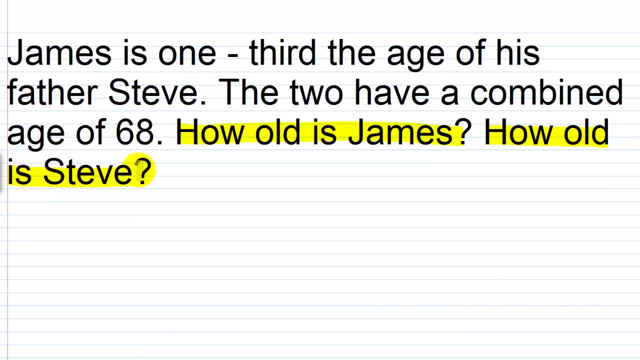 old is Steve. So we don't know their age individually, but we do know the combined age, it's 68. So this is kind of a typical problem where we know the sum of the quantities, but we don't know the individual quantity. So that means aught of the unknown is � suspension 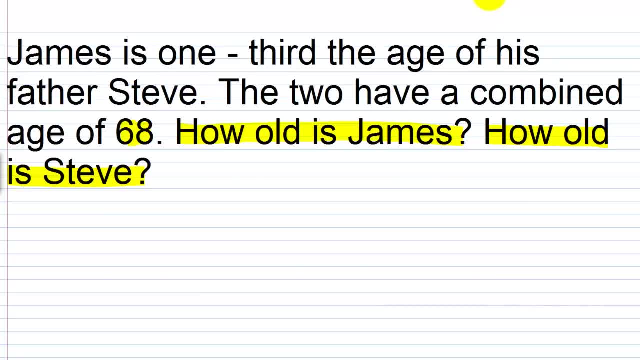 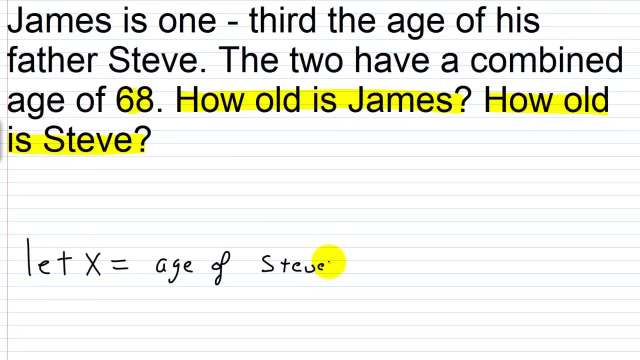 or equal toд, but the individual quantity is not known. Let's start by assigning a variable to represent one of the unknown. Let's let x equal the age of either James or Steve, it doesn't matter, Let's say Steve. So let's let x equal the age of Steve. We. 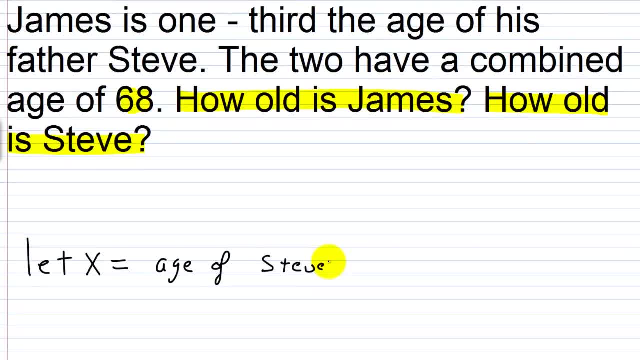 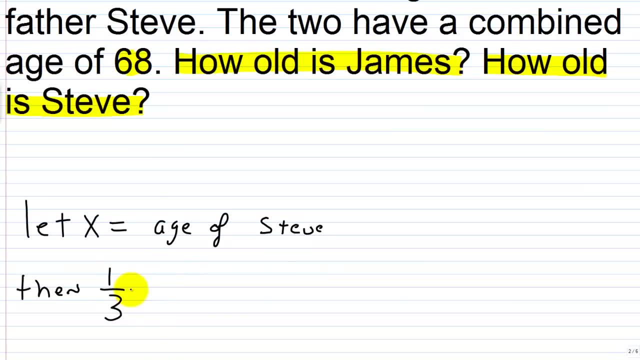 know that James is one-third the age of Steve. so that means that we can say then, one-third times the age of Steve is one-third加 all. 곶基金 fo st noite avantломarle. If we times the age of Steve, which is x, would be equal to the age of James. Very, very easy. 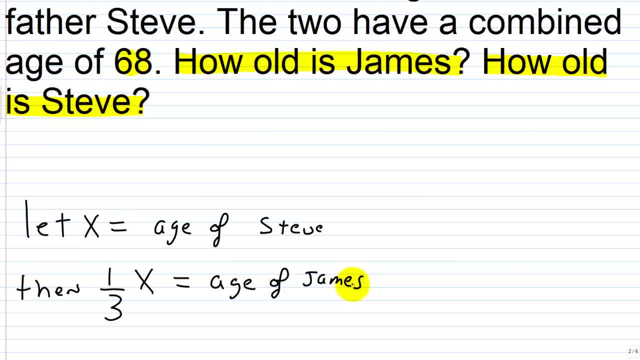 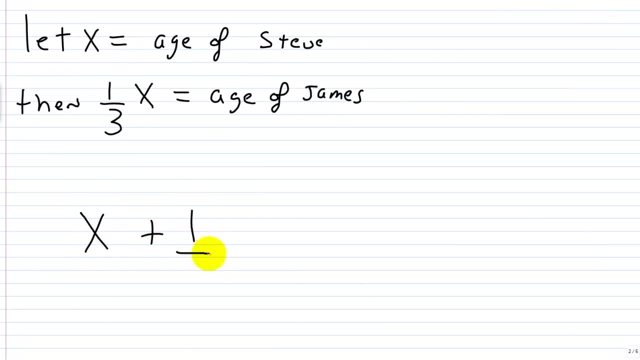 Okay. so to make an equation, remember that the age of Steve plus the age of James, which we have x and one-third x, if we add those two amounts together, it gives us 68. Told that in the problem, So let's do that. We'll have x plus one-third x equals 68. And if 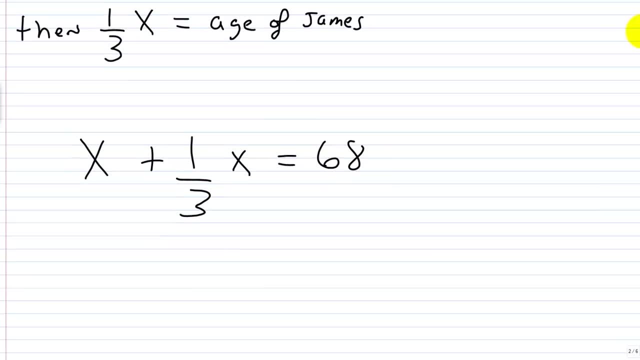 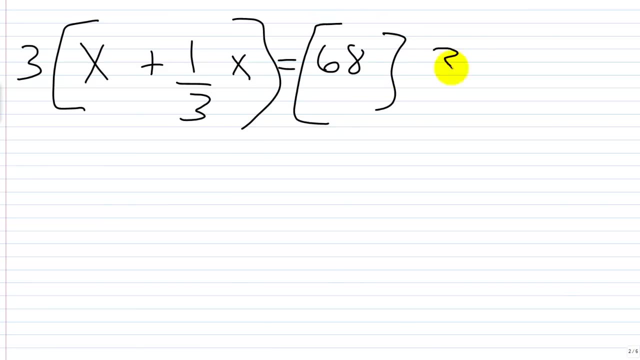 I want to clear this fraction here. I can just multiply both sides of the equation by three, So I'll have three times this side and three times this side. So we'll have 3x plus x equals 204.. 3x plus x is 4x, So I'll have 4x equals 204.. And we'll divide that. 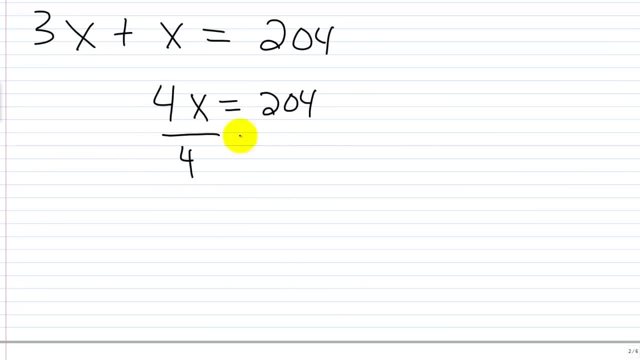 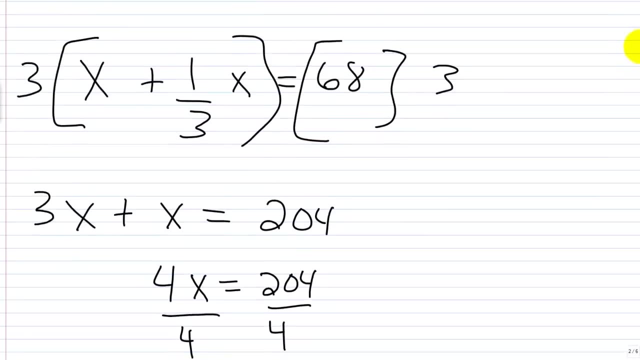 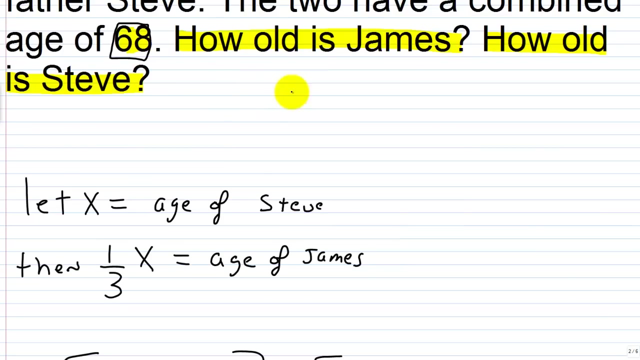 both sides of the equation by 4 to get x. by itself We get x equals 51. So let's scroll back up and interpret that, because we're not done. So x is the age of Steve. Okay, Steve is the father. So how old is Steve? Steve is 51 years old Now. hold is James Well. 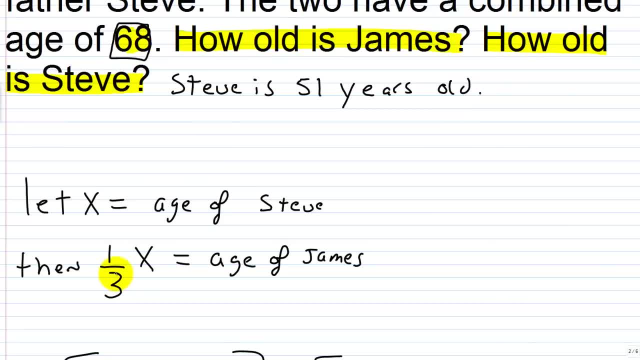 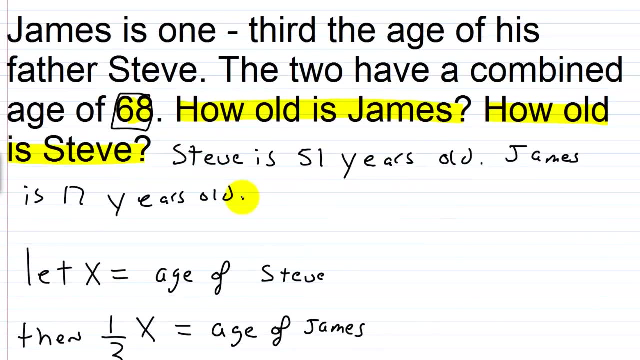 James is a third of the age of Steve. So James is 17 years old And this is completely consistent with our problem. You can see that James is one-third the age of Steve. Right 17 is one-third of 51. And we can also see: 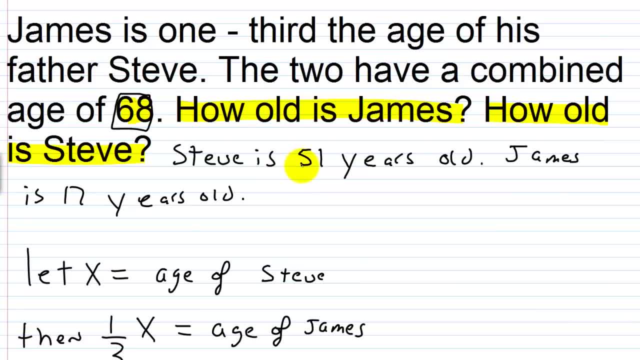 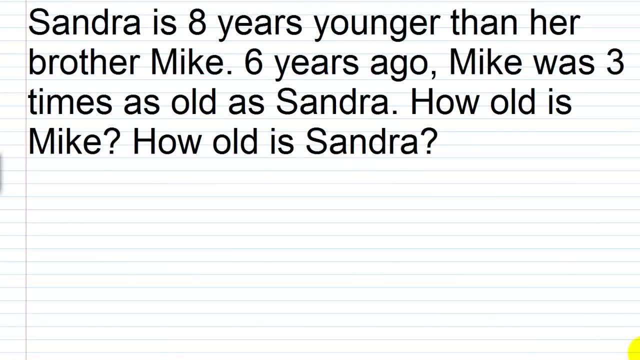 that 17 plus 51, the combined age would be 68. Okay, 51 plus 17 is 68.. Let's take a look at another one. So Sandra is eight years younger than her brother, Mike. Six years ago, Mike was three times as old as Sandra. How old is Mike? How old is Sandra? 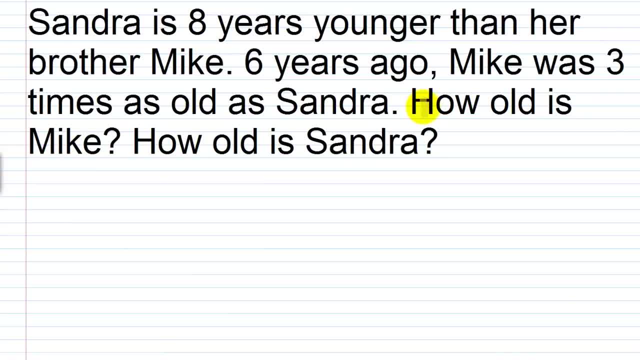 So again we are asked for the age of each individual. How old is Mike? How old is Sandra? One thing that's different is we're not told their combined age. So we have to find another way to set up an equation. But before we get to that, let's let a variable, let's say x. 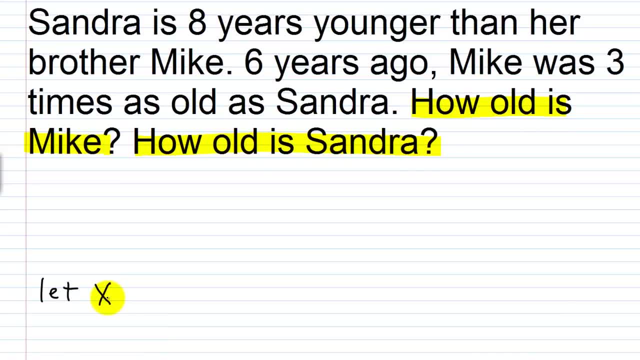 equal the age of either Mike or Sandra. It doesn't matter which one, Let's say Sandra. So let x equal Sandra's age And it says that Sandra is eight years younger than her brother Mike. So if I take Sandra's age, okay, and 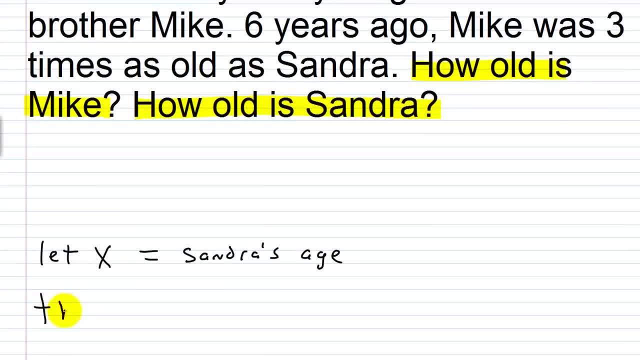 I add eight years to that, or x plus eight, I should get Mike's age. So this is Mike's age. Okay, So we've modeled this. We have Sandra's age and we have Mike's age, But how are we gonna set up an equation? 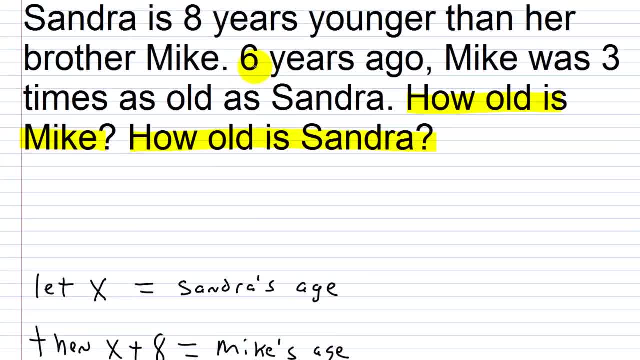 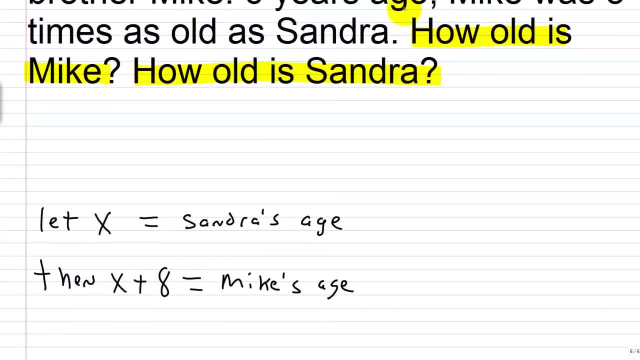 We don't know the combined amount, We've got to keep reading. It says that six years ago Mike was three times as old as Sandra, So six years ago. If I think about Sandra's age six years ago, it would be x minus six. So this is Sandra's age six years ago. And if 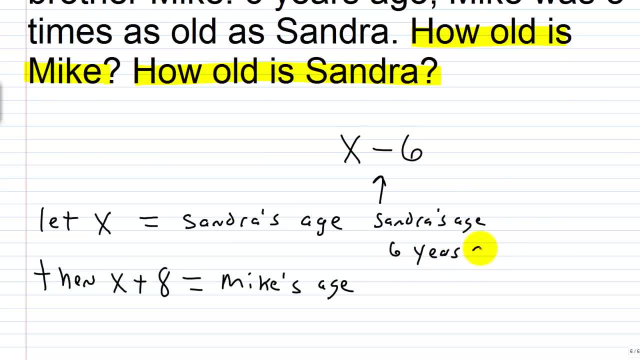 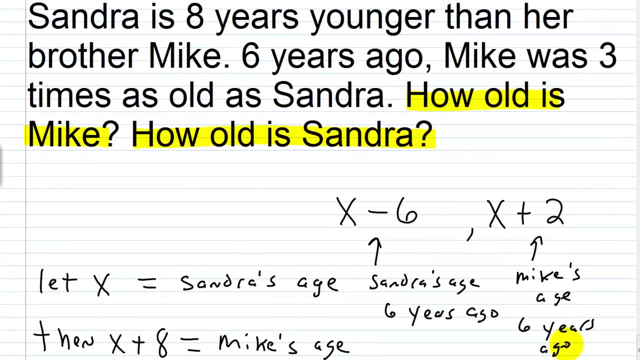 I think about Mike's age six years ago. it would be ten years ago Six years ago, So six years ago. X plus 8 minus 6. if I simplify that, it would just be X plus 2. so X plus 2 would be Mike's age six years ago. so let's think about this. 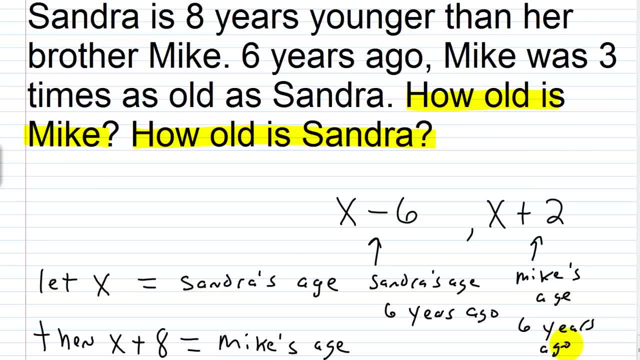 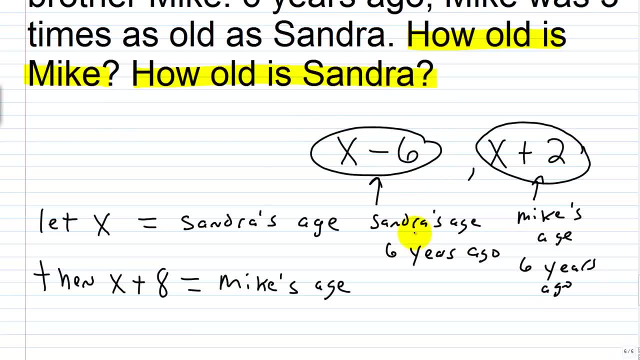 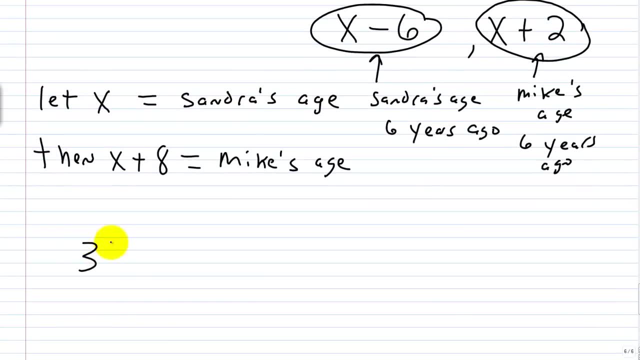 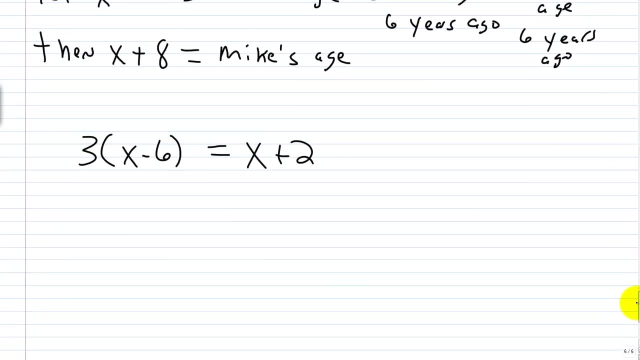 again, six years ago, Mike was three times as old as Sandra, so I know that Mike's age here is three times this amount which is Sandra's age. again, this is in terms of six years ago. so that means that three times this quantity here, X minus six, is equal to X plus two. now let's kind of cover this again, and I 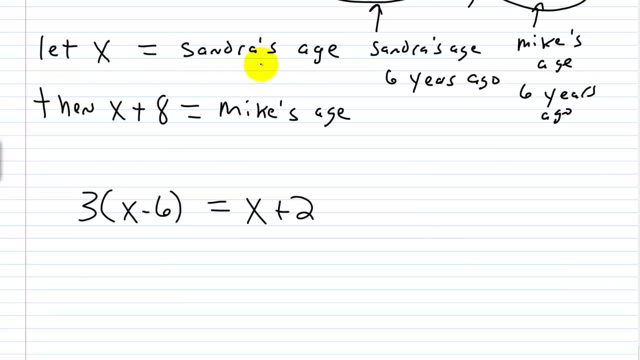 know some of you will be lost. in the current time period, X is Sandra's age, so that means six years ago she was X minus six. this is six years ago ago. Currently, Mike is x plus 8 years old. Okay, that's his age. 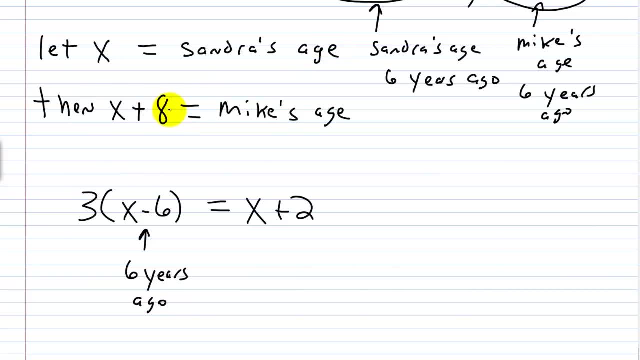 Because we took Sandra's age, we added 8 to that to get Mike's age, Now, 6 years ago. we subtract away 6 from this, we get x plus 2. This is 6 years ago And in the problem we're told that. 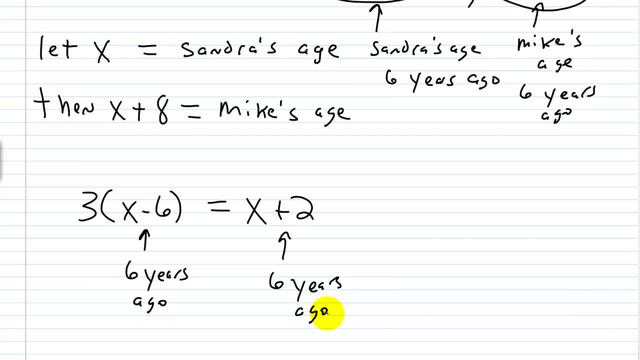 6 years ago, Mike was 3 times as old as Sandra. So, in terms of 6 years ago, 3 times the age of Sandra 6 years ago- this is her age 6 years ago- is equal to Mike's age 6 years ago, which is x plus 2.. 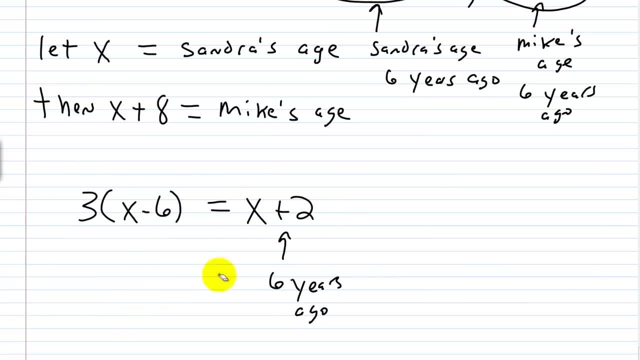 So what we're going to do is we're going to solve this for x and we're going to find out the current age of Sandra. So 3 times x is 3x minus 3 times 6,, that's 18,. 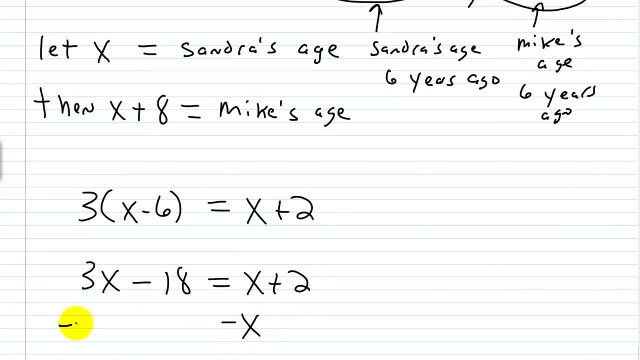 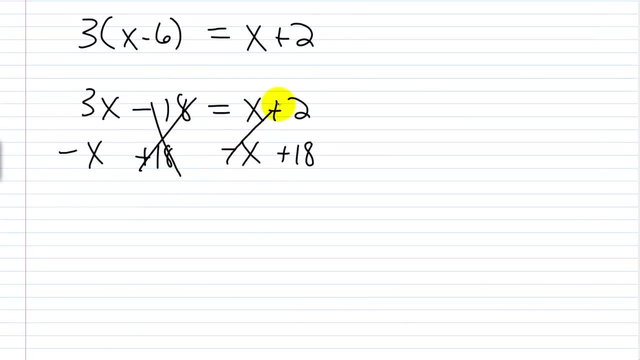 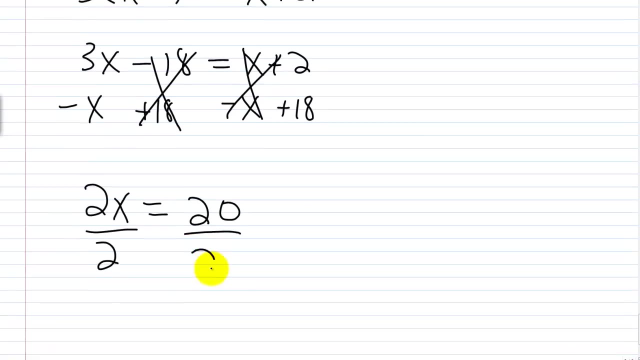 equals x plus 2.. Subtract x away from each side. add 18 to both sides. So this is gone and this is gone I'll have. 2x is equal to 2 plus 18 is 20,. divide both sides by 2,. 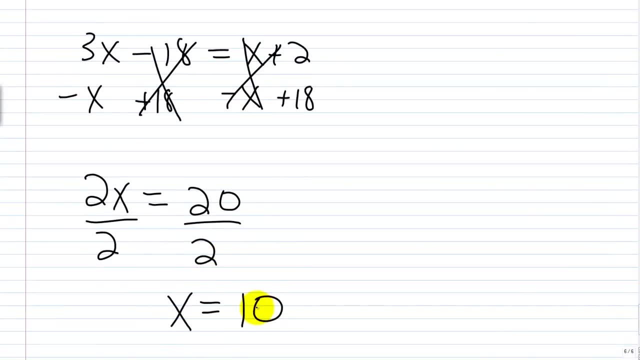 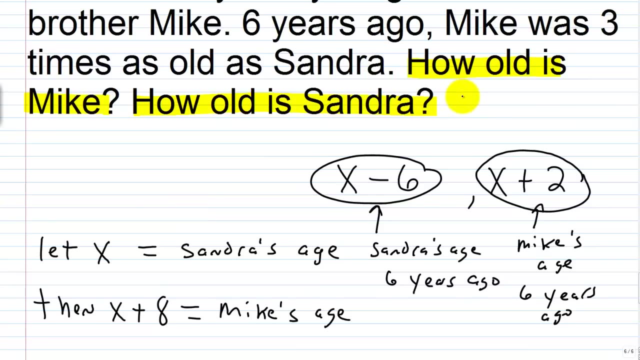 and I get x equals 10.. So I know what Sandra's current age is now, Because, again, x is equal to Sandra's current age. So to answer this, we'll say that Sandra is 10 years old And Mike, remember, he's 8 years older.